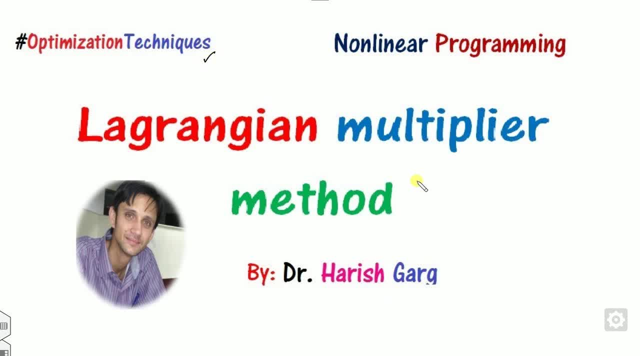 Hello everyone, welcome to the next lecture on the optimization technique. Today we will discuss about what is the Lagrangian multiplied method and how we can solve this non-linear programming problem with the help of this. Myself, Dr Gaur, working in the School of Mathematics. 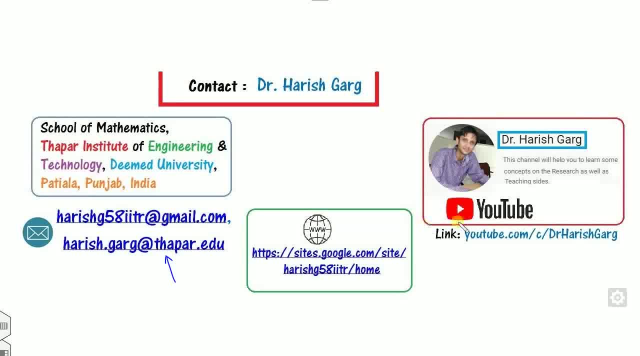 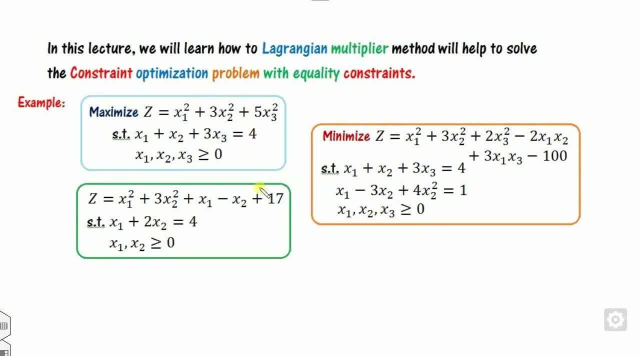 Thapar Institute, India. You can contact me through either of my email ids or through my channel, this one. What is the task of this lecture is? we will see how we can solve such type of the problem. You can see, this is the constraint optimization problem, in which the first example 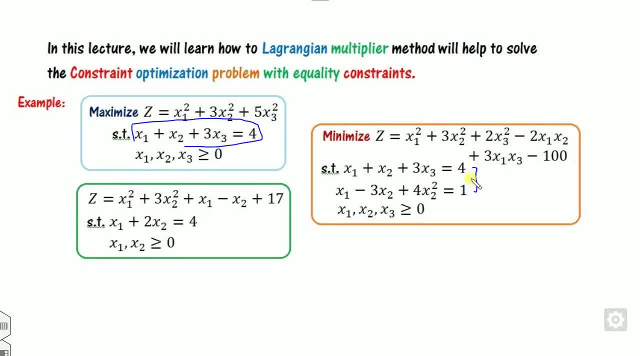 say it is only the one constraint. This one has the two constraints. Second one is a non-linear, while third one is also with a linear one. So, and the major question arises here is this method that is we will discuss in this lecture, is applicable only when the constraints are. 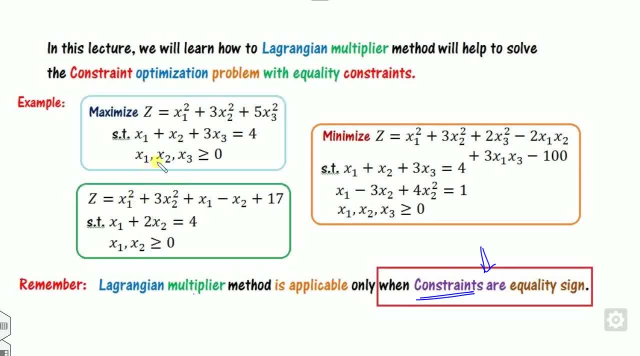 equality sign. So what we will discuss in this class is: we will see how we can solve the problems related to the first problem. So what we will discuss in this class is: we will see how we can solve the problems. and third, while in this case there are the two constraints, So we will see this in our next. 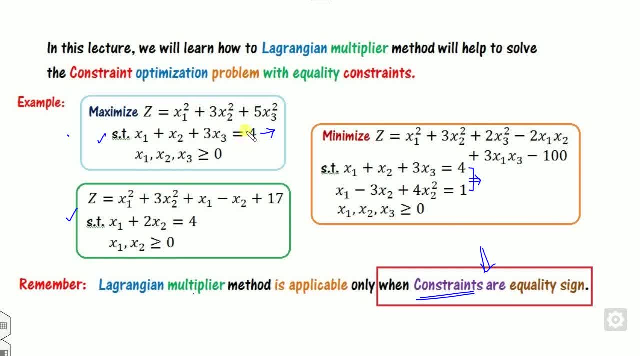 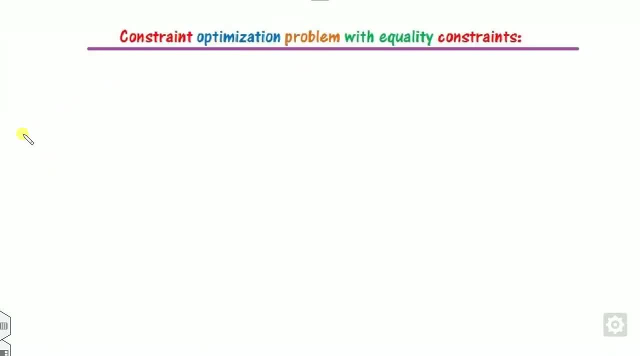 class. But right now we will discuss that how we can solve the problems having one constraint. So the first question arises is: what is the constraint optimization problem? So any problem which is written in this form: maximize or minimize the function subjected to these constraints we call as the constraint optimization problem, with. 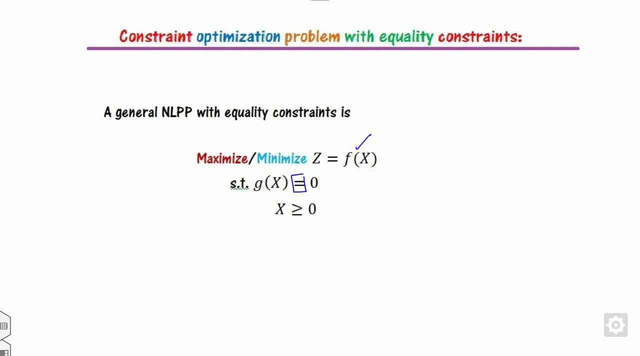 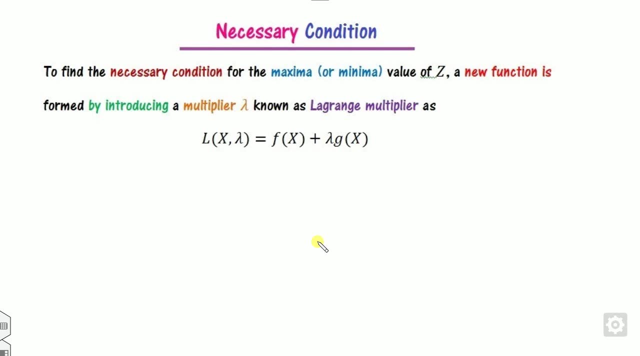 equality sign. Make sure that the function f and the function g are both differentiable with respect to x. Once you have this, then what is the necessary condition for the existence of maxima and minima? For this we have defined the new function, that is. 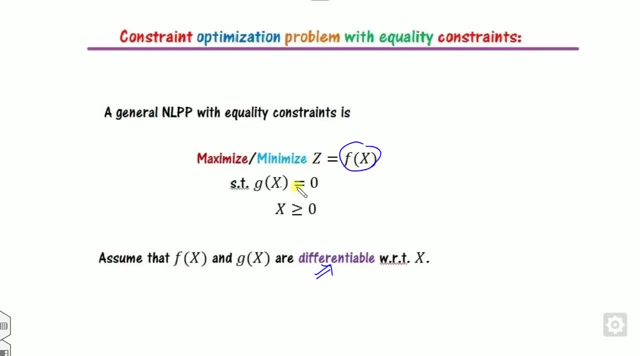 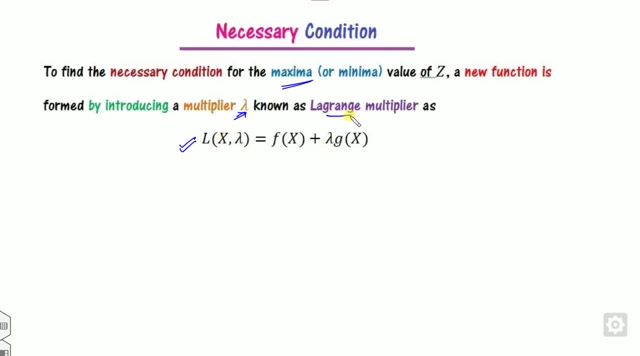 l, which are based on this f of x and as well as the g of x, and we can combine them with the help of this lambda which is called as the Lagrange multiplier, And this Lagrange multiplier is the unrestricted in sign. What is the meaning of this is you can define like this way, or you can define: 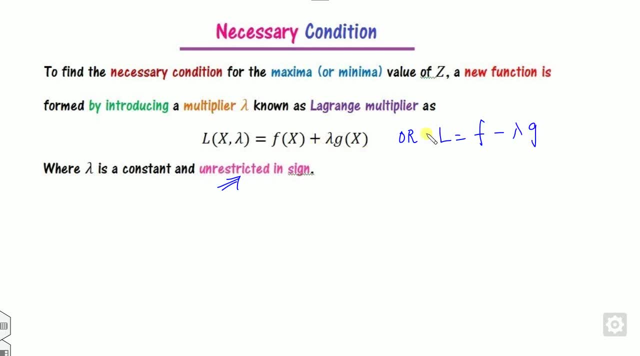 the l in terms of this. that is, either you can use the plus or minus. this does not mean any of things. So lambda is unrestricted, means it has either the positive or the negative value, And the function l is called as the Lagrange function, with Lagrange multiplier: lambda. 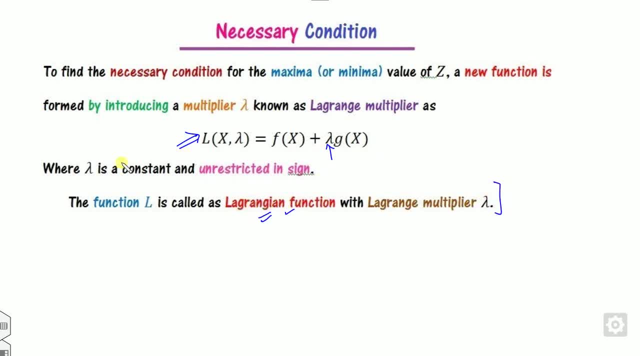 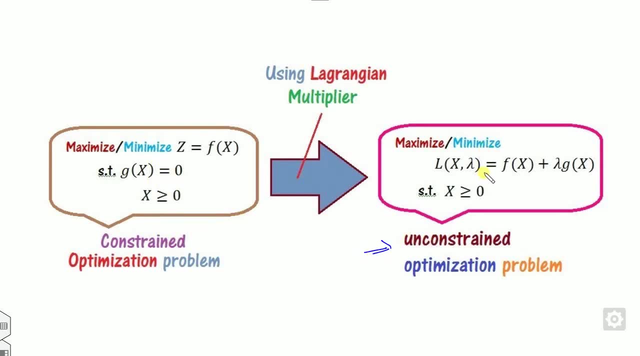 What is the purpose of doing this? why we studied this Lagrange multiplier is the main purpose is that for any constraint optimization problem, we can convert into the unconstrained optimization problem with the help of this Lagrange multiplier lambda. once you are the unconstrained optimization problem, then all of 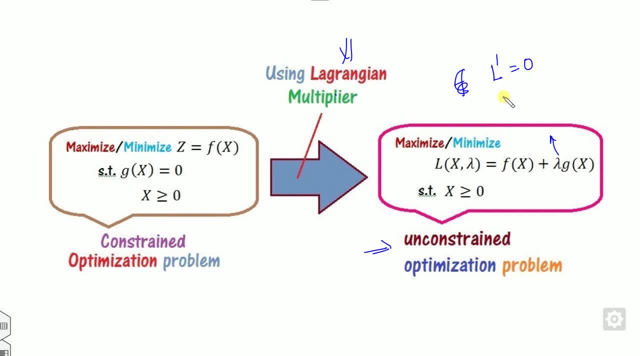 you know that. how you can find the maxima and minima is there: first derivative should be 0. second derivative, less than or greater than will be 0. we can find the maximum or minimum. So the necessary condition for the existence of the maxima, minimum will be. 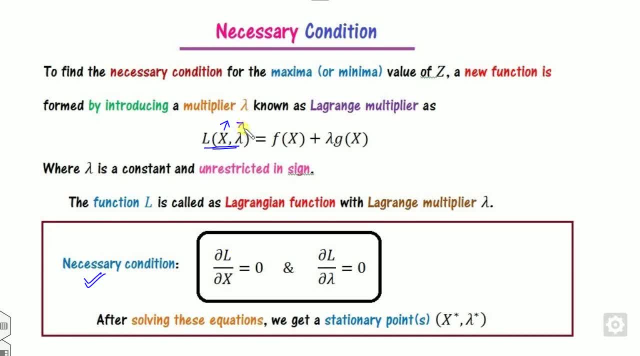 here there are the two parameters. one is the x and second is a parameter. So we can take the partial derivative. with respect to x is 0 and with respect to lambda. After solving this, we will be able to find the maximum and minimum. So we can take the partial. 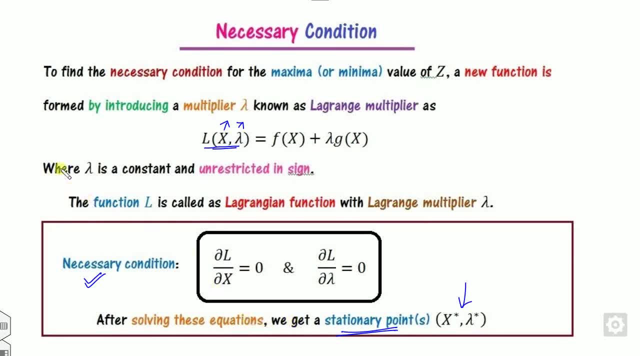 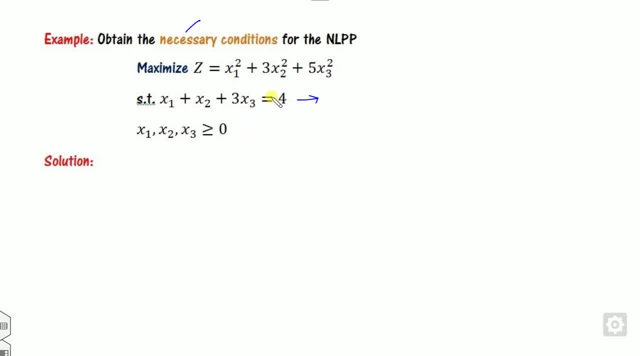 derivative with respect to x is 0 and with respect to lambda. After solving this, we will be able to get the sum point, called as the stationary point. For example, if I say: write the necessary condition for this nonlinear, and you can see, this is only one constraint which have the equality sign. 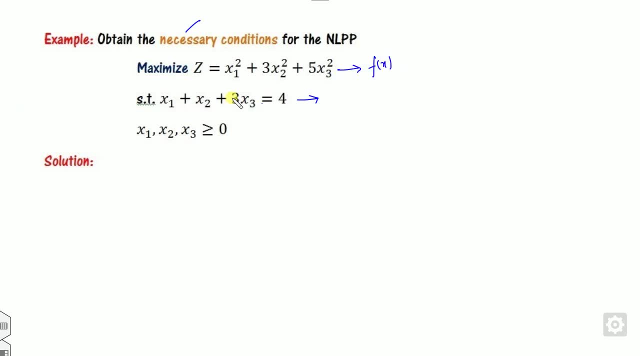 So this is my f of x, this is my g, so we can define the Lagrange multiplier. that is, this is my f plus, or you can take a negative also. So what is the necessary condition is we can. how many variables are there? x1, x2, x3 and the fourth one is lambda. So the necessary condition 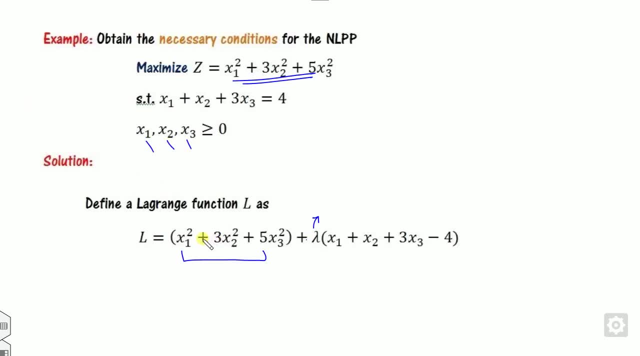 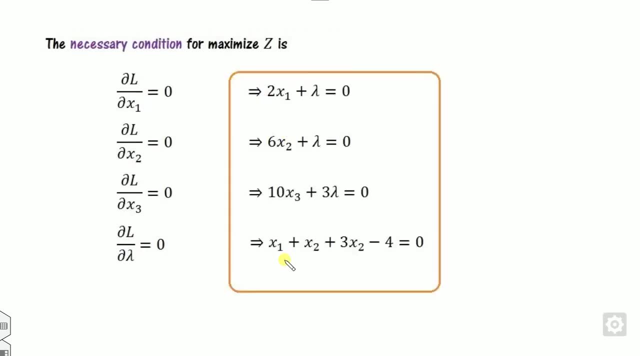 will be here. what is the partial derivative with respect to x1 is? you can take as a 2x1 and this is plus of lambda. Similarly, you can define the other side. So, based on these four equations, you can find the values of x1, x2, x3 and lambda easily. How you can see from here you can. 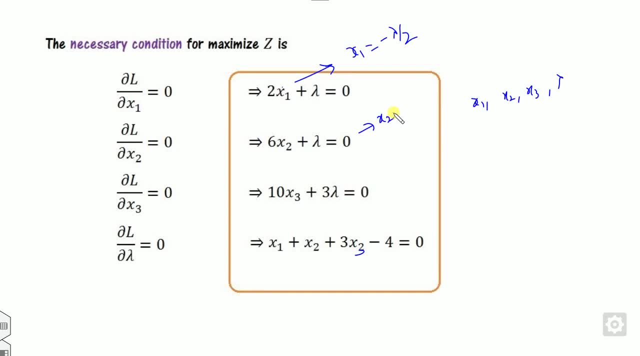 find the value of x1. from here you can find the value of x2, from here you can find the value of x3. from here you can find the value of x2, from here you can find the value of x3. and if you substitute all values here, you will get the value of Lambda, and hence you will get here. 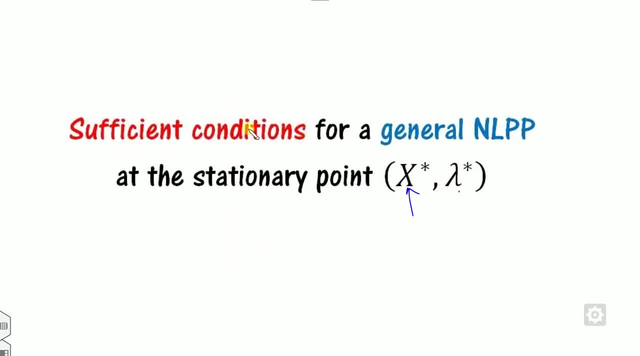 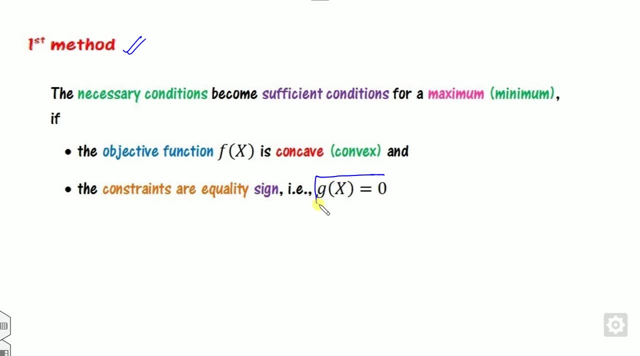 Now, once you are finding this point, that is, X star and Y lambda star, then what is that? sufficient conditions are there. we are discussed the two method. first method is: if the constraints are equality sign, then these necessary condition becomes the sufficient condition provided. if your objective function is maximization, then you have to prove that the function is. 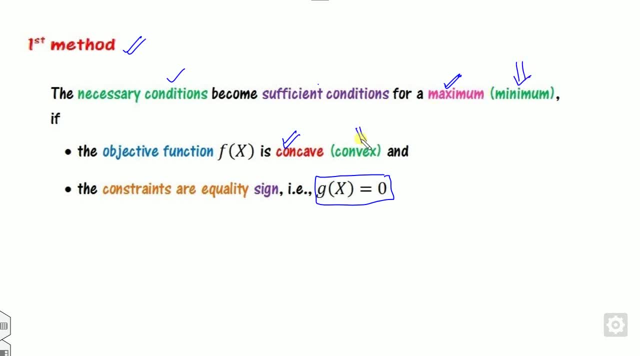 concave. if your problem is minimization, then you have to prove that the function is convex and how we can prove the convection concave that we have discussed in our last lecture. that is based on this principal minor speed. So you can watch the last lecture related to the convection concave function. second, 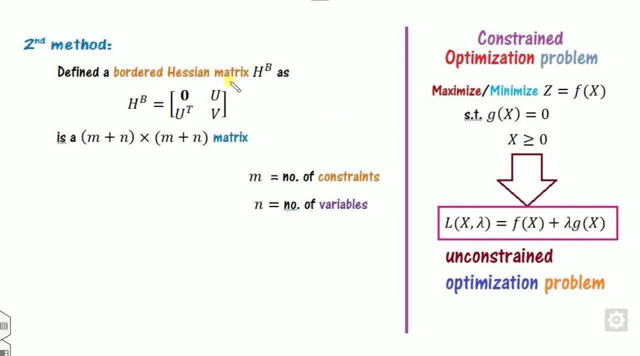 method is that, once you are converting the constraint problem into unconstraint, you have defined the border Hessian matrix HB, which are defined like this way here: M is the number of the constraint, N is the number of the variables, And the size of this will be M plus N, M plus N. once you are writing this, then what is the? 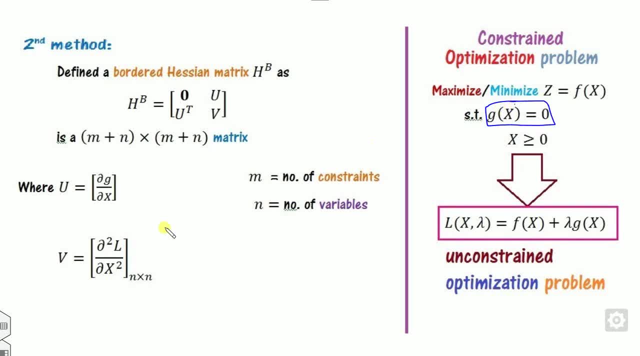 U is nothing but the partial derivative of this constraint and V is nothing but the partial derivative of this L. So you can see what is the partial derivative of G is nothing but X1 up to Xn. and the second derivative, this is the Hessian matrix, so we can define. 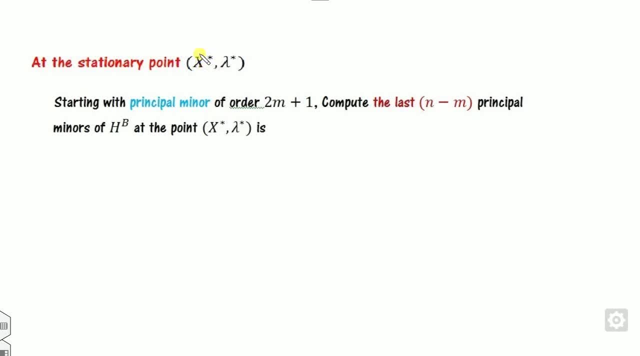 like this way. So once you are finding this stationary point, then we will check the maximum or minimum depending upon the sign of this, If they are alternating sign or the other same sign. So we are discuss this with the help of the numerical example here. 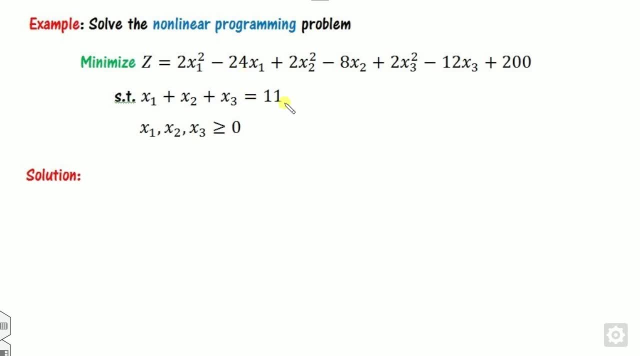 So first of all, look at that. the constraints is my single, So there is a one constant. So your first task is to define this Lagrange multiplier, that is a. L is equal to F plus G times of this. How many variables are there? 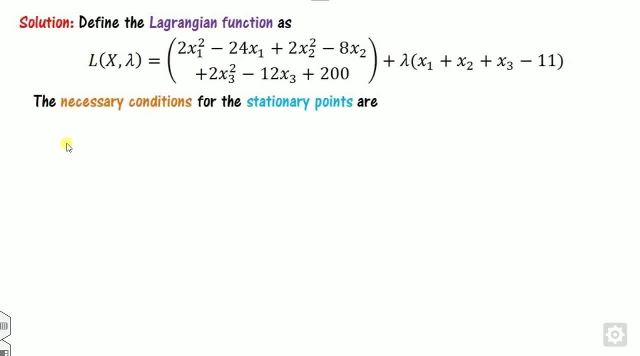 This is the X and lambda, so we can define the necessary conditions as of this. So what is the partial derivative of this L with respect to X1.. You can easily find all this one. So, in order to find the value of the X1, X2, X3 and lambda, or you can call a stationary, 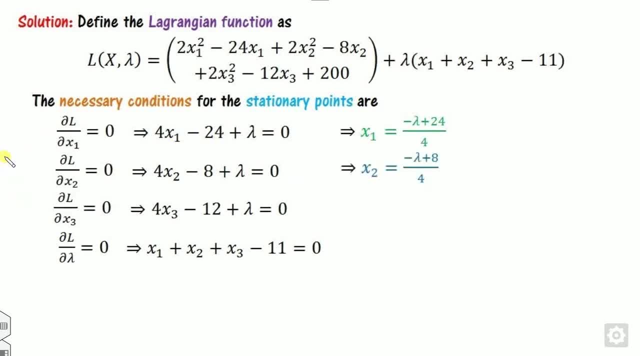 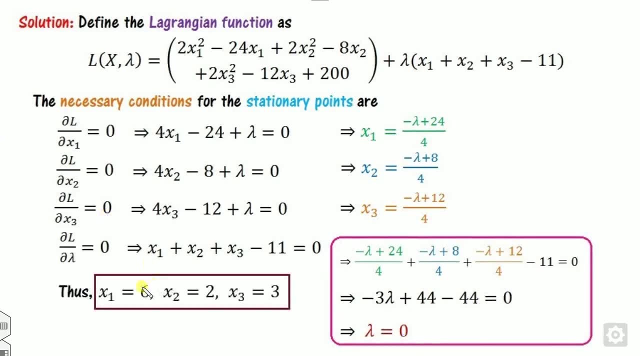 point we can find the value of X1 from the first equation, X2 from the second equation. third is: there We can substitute all this value. in here we will get the value of lambda as a 0. So therefore, once lambda is 0, we can substitute. here we can get the X1, X2 and X3. 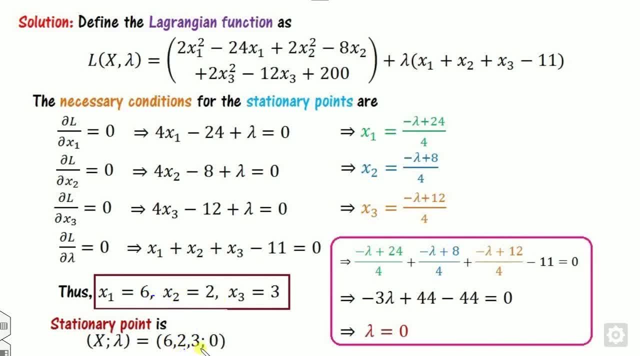 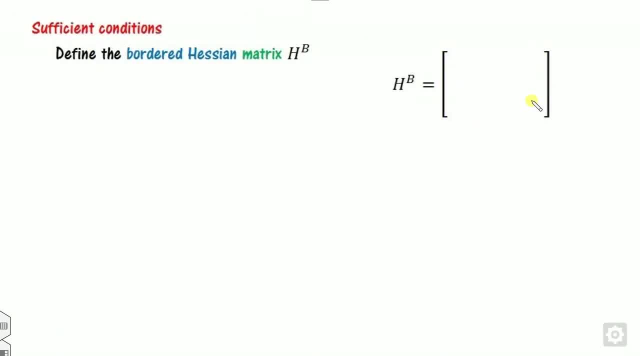 Therefore, the stationary point will be X1- X3.. To check whether this point is the maximum or minimum of the function, we can define the Hessian matrix. What is that? in order to define this, firstly, we have to identify what is the size of this. 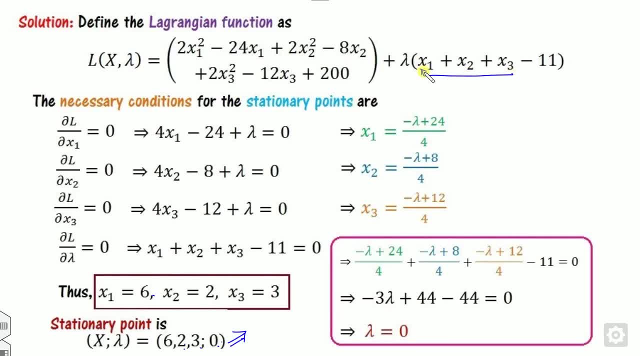 What is the M is number of the constraints. how many constraints are there? only one, So M will be my one. What is the N is number of the decision variables: X1, X2, X3.. So N will be my three, So you can define like here. 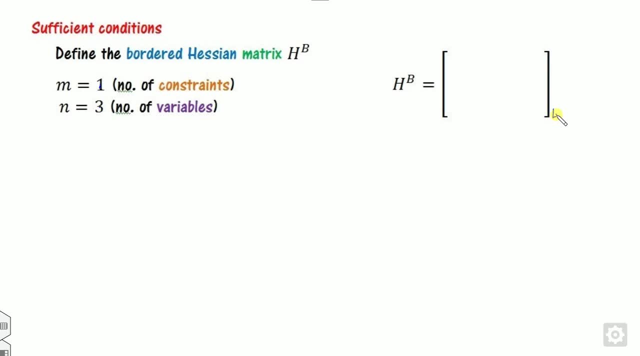 So therefore, The size of this will be M plus N, So it will be my four cross four. So therefore you have to define like this: What is the U is that is a partial derivative of G with respect to X. So how many G are there? what is my constant is X1 plus X2 plus X3 minus 11.. 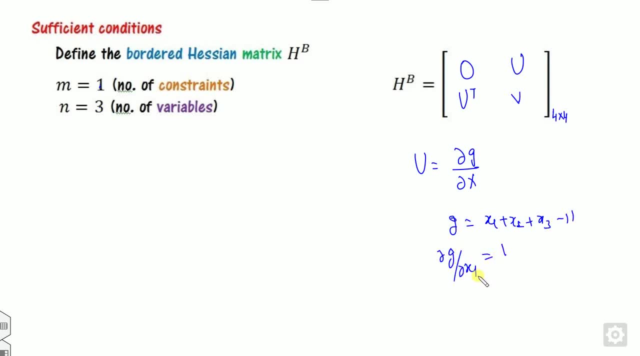 What is the partial derivative of G with respect to X1 is 1, with respect to X2 is also 1, X3 is also 1.. So this is my 1, 1, 1.. And here is 1, 1, 1.. 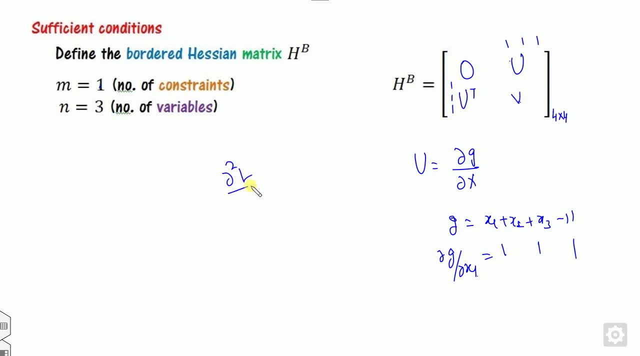 What is? the V is partial derivative of L with respect to the X is. So we can define like here: Because what is that? this is this one second is X1, X2 and so on. So this is it. Now you can define the principal minus. 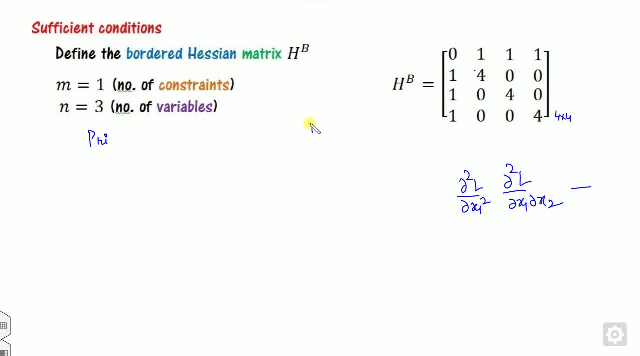 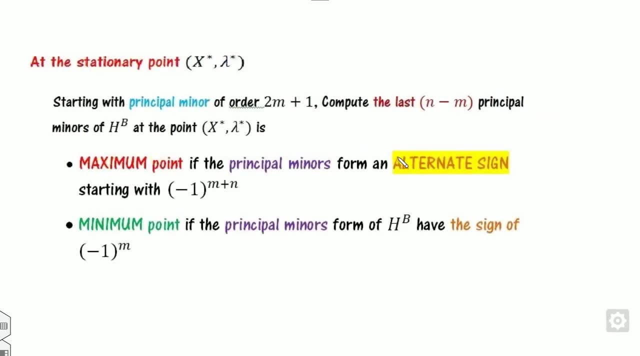 Now the size of this is 4 cross 4.. So how many principal minus are there? 4, D1, D2, D3 and D4. but instead of finding all those principal minor, We will start the principal minus of 2m plus 1 and n minus m. 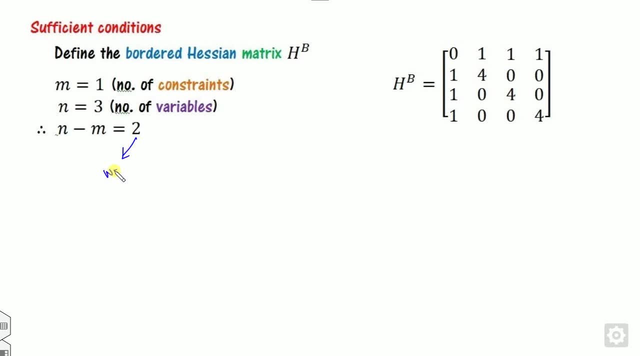 So what is the value of the n? so it this will give you. we have to calculate two minus, We have to calculate the two minus. But what are those two minus? is it D1 and D2, is it D1 and D3, and so on? 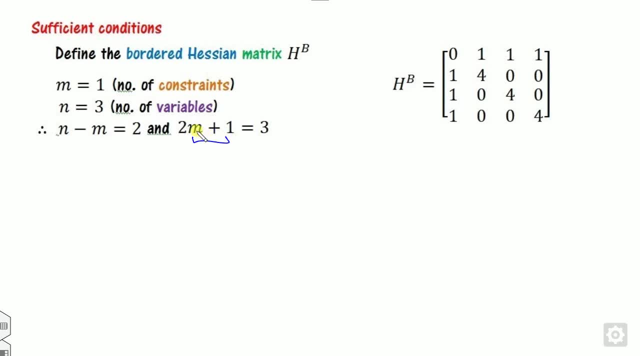 So that will tell us about the 2m plus 1.. So what is the value of the 2m plus 1 is 3. it means we will start the principal minus from the D3. what is the number is here, and the next one is the D4. what is the D3? is we? 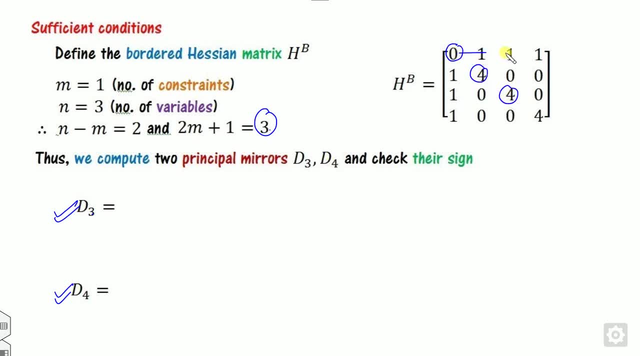 have to take the first three diagonal entries and the corresponding minor will be here. So this is my D3. we can calculate the determinant of this. similarly, we will calculate the fourth is there. So what is the determinant of this? and here we will calculate it's a negative. and second, 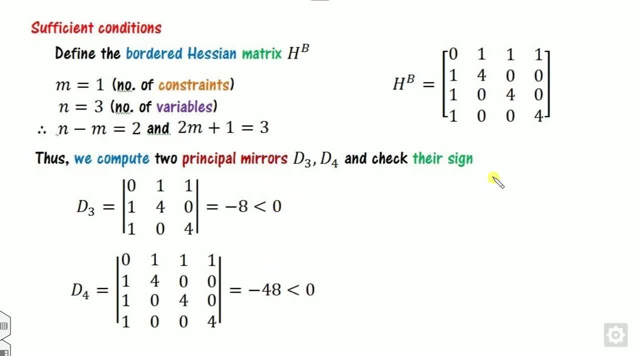 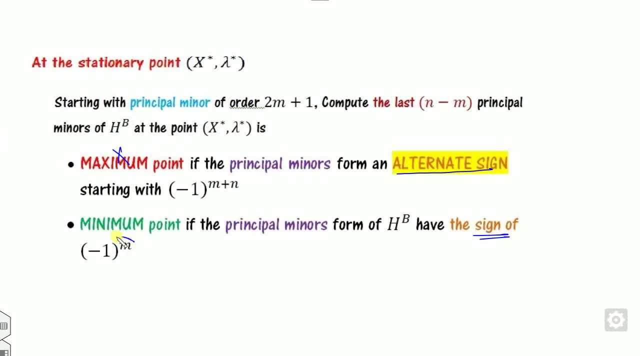 one is also negative. Now the point X star. what is the stationary point? is the minimum or maximum you can see? are the alternating sign? no, it means it will not be the maximum. are they same sign? yes, it is the same sign. but if the same sign is of this nature, what is the value of the m? 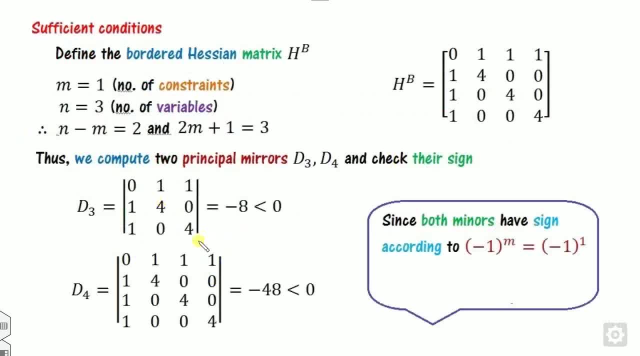 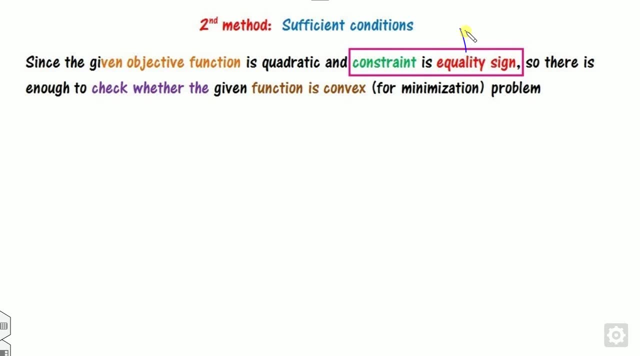 here is 1, so are they both negative? yes, so, since both have the same sign. so therefore, this point is my minimum point. hence the stationary point is my minimum. Second method is: there is no need to find the border Hessian matrix, you can simply, since 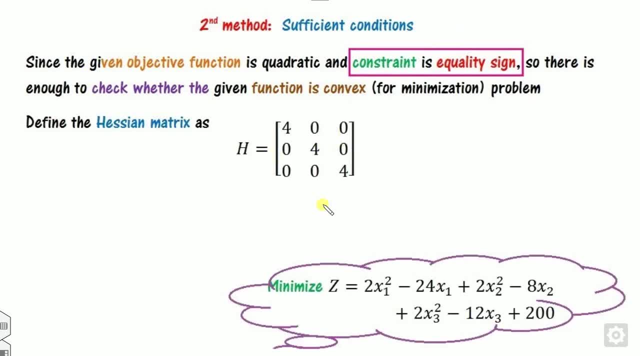 the equality signs are constants are equality, so you can define simply Hessian matrix here for this Z. so if I call as this as F, so how you define that: this is X1 square, this is X1, X2, and so on. so this is 3 by 3. now you can define the principal minor 1, 2 and 3 as: 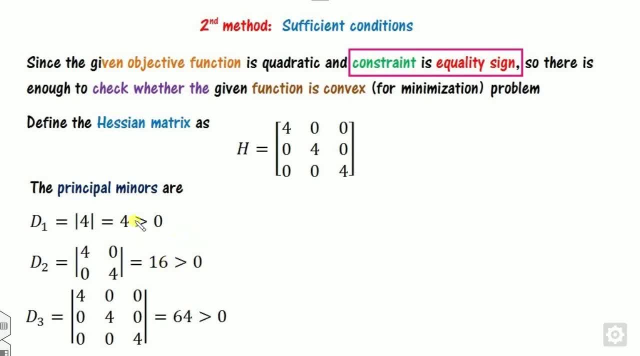 follows, since all are the greater than 0. so we can say this is the positive definite. hence it's a convex set, convex function, so it give a minimum. Also, you can see That what are the eigen values of this? the eigen values of this are 4, 4 and 4 and both. 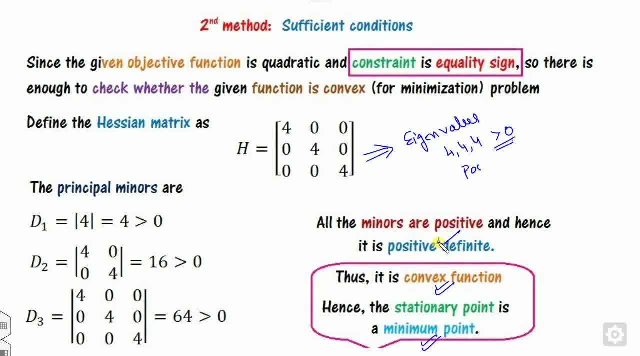 all are greater than 0, so it means this is again a positive definite, hence it's a convex function. so therefore is a minimum point. so you can take any one of method, the result will be same. look at the second example. we will apply the same method to all those problems. 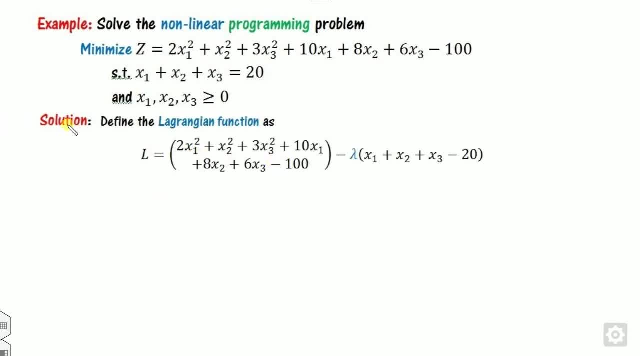 again, one constant is there. we will define the L now. this time I have taken the negative sign, So you can take either as a plus or negative, there is no problem. so you have to find the necessary condition. firstly, you have to take this from the first one. you have to find the. 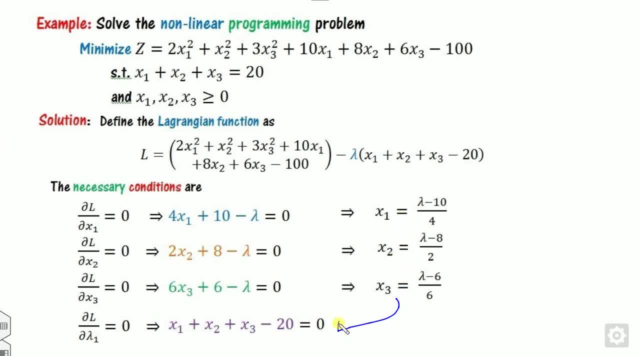 value of X1, second X2 and X3. after this you can substitute the value here. you will get the value as 30. once you will get lambda as a 30, you can substitute the value here. so it will be my 20 by 4, it will be my 22 by 2, it is my 24 by 6. so the answer are 10- 11. 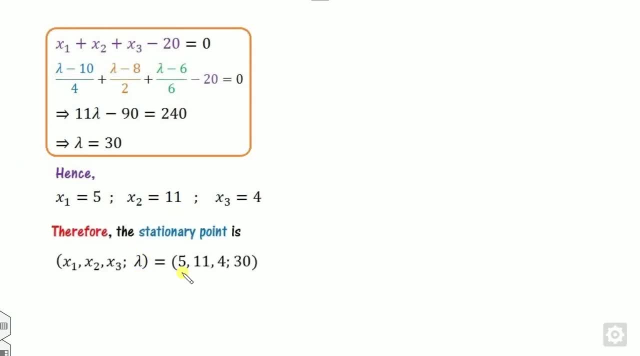 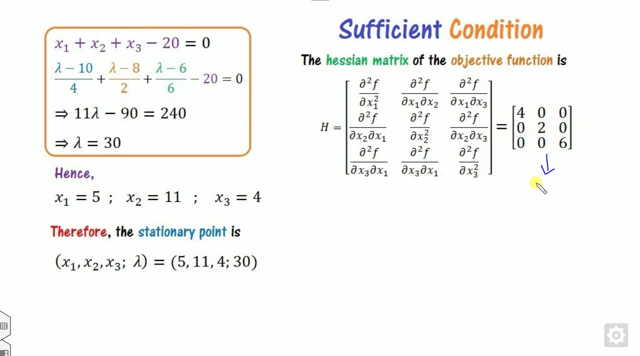 and 4.. So, therefore, stationary point is my here. now check whether this stationary point is a maximum or minimum. we will define either the border Hessian matrix or else, since there is a one constraint, so we can define the H simply as here. and what are the eigen values of this? 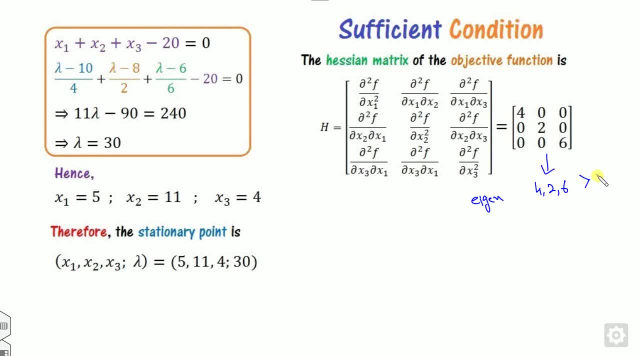 eigen values are my 2, 4 and 6. both all are positive, so it means this is the positive definite. hence this is the convex function. so once it's a convex function, so it always gives a Minimum. otherwise we can also find the principal minus the first principle, minus second and 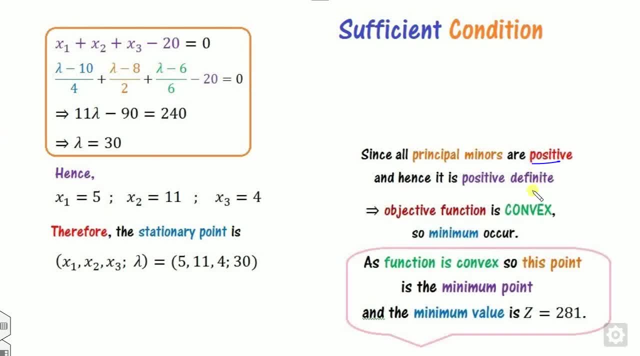 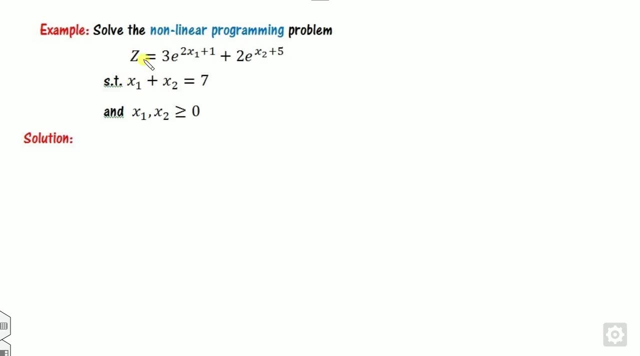 third, all are greater than 0, so therefore we can say this is the convex function, so the minimum occur. hence this point is the minimum point and the value of the Z is 281. similarly, look at the third example and if you clearly see what about the third example? 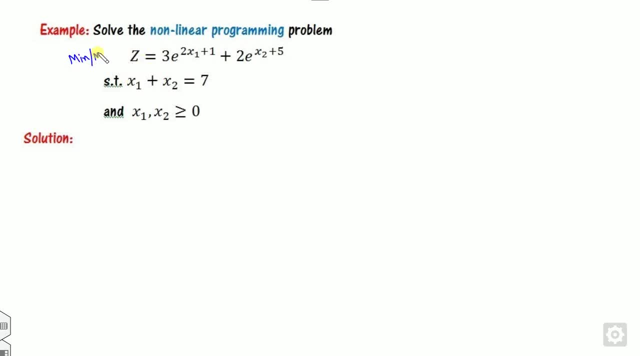 is. look at the. what is that? it is neither the maximum nor the minimum. so what is the question about that? Can you find the minimum or maximum of this function? so, in order to check, firstly, what is the minimum or maximum, you have to define their convexity or concavity. if you prove that, 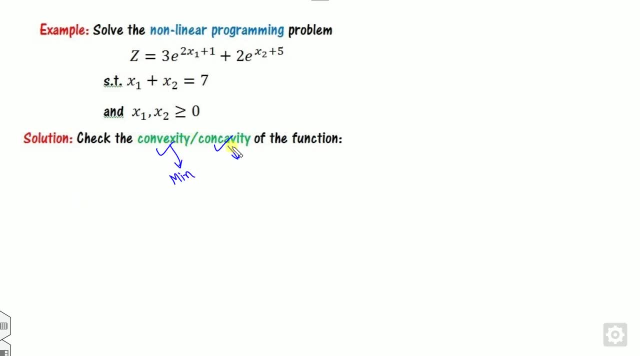 the function is convex, then it's a minimum. if you prove that this is concave, then it is a maximum. so how you check that? we already discussed that. we will define their Hessian matrix, so we will start with the Hessian matrix of this, since there are the two variables. 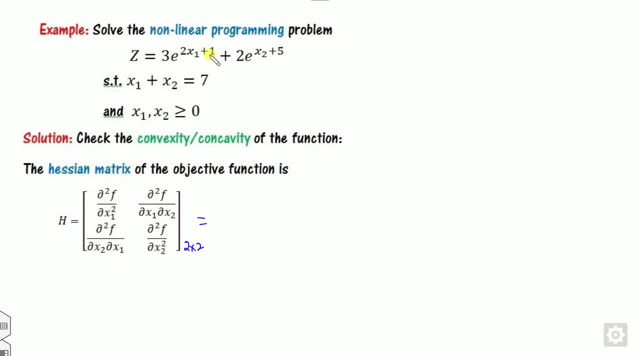 so it will be that 2 cross 2.. So what is the second derivative of this? This with respect to x1, it will give you here and so on. Now you can find the principal minor. what is the first principal minor is? it is always. 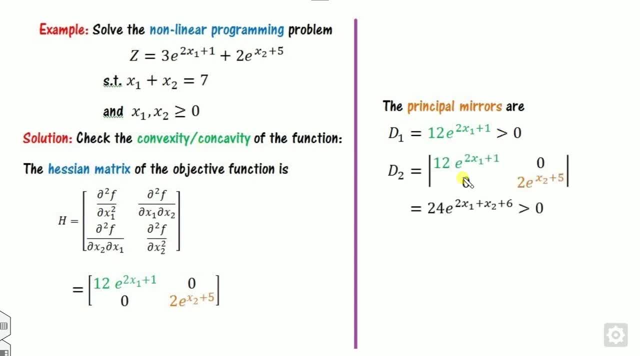 be greater than 0, because x1 and x2 both are greater than 0. second principal minor is this: again, these are greater than 0. so since both the principal minus are greater than 0, so it means this, the positive definite. hence this is the convex function, therefore minimum. 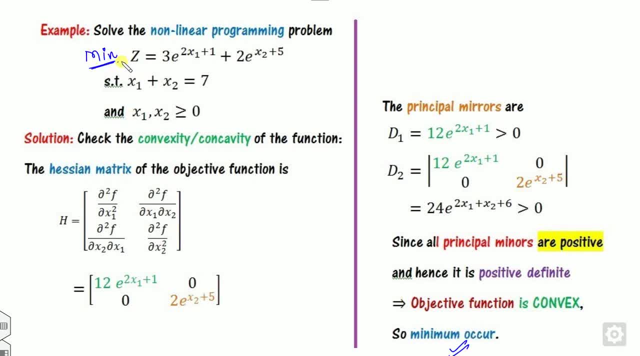 occurs. so that is this problem is minimization, and since this is the convex function, so we already knows that for every local implies the global is there in the convex problem. so therefore this sufficient condition are automatically satisfied, so we need only to check what is the point. so therefore we have to define their necessary condition of the 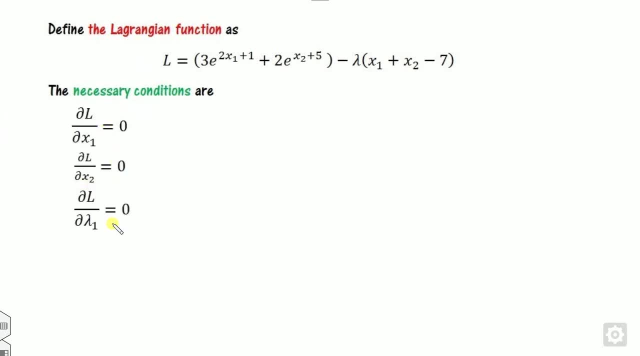 end. so what are the necessary condition we have to take that? this one. so this is. there is only one, so we can take us here. what is the derivative of this with respect to x1? so it will be this one. So, from these three equations, 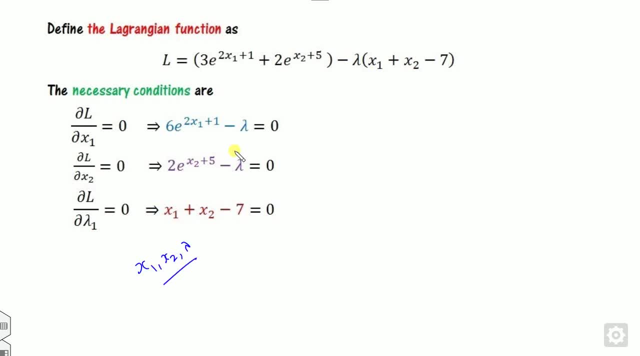 You have To find the value of x1, x2 and lambda. so from here you can find easily the value of lambda. so says both are equal. so it means you can equate them. I can calculate the value of x2 from here: 7 minus x1. I can substitute the value of here and after the solving you will. 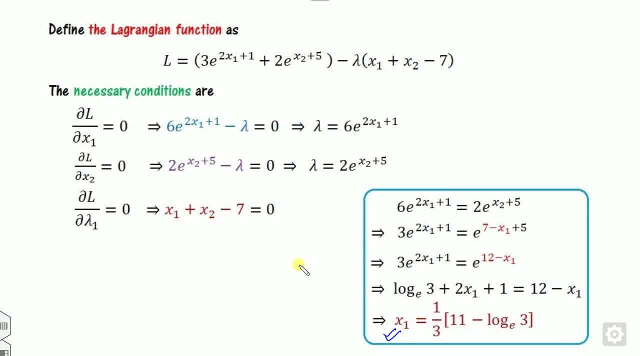 get x1. is this so, once x2 will be here- x1 is here, so you can find the value of x2- will be this: that is here, so x1 and x2 will be here. you can substitute the value of x1 and you can substitute the value either in this or this. you will get the value of lambda. 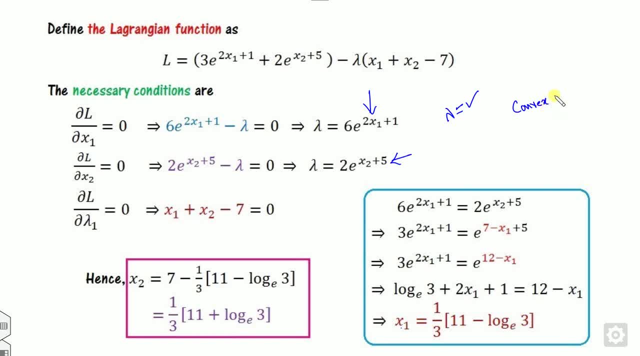 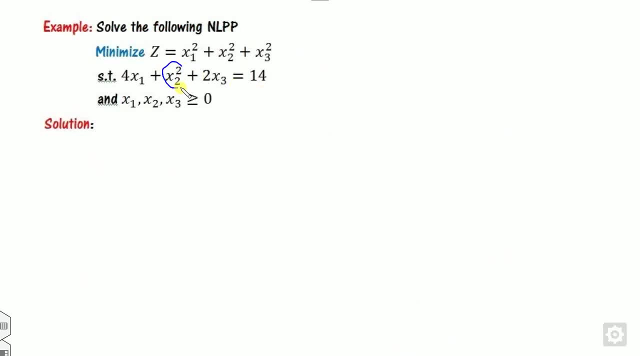 and since in the previous we already proved that this function is convex, set convex function. so therefore the point x1, x2, this is x1, this is the x2 are my minimum point. look at one more example. in this case you can see this is a nonlinear, but the constant is only one. 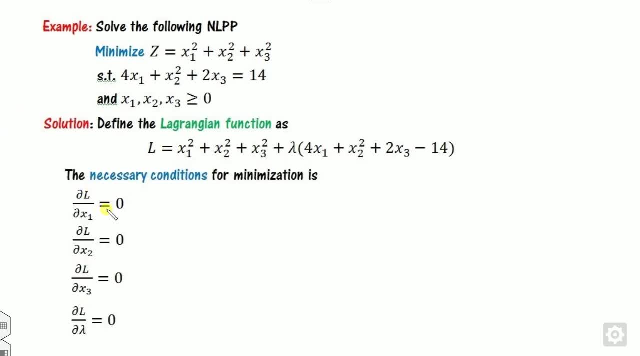 so you have to firstly define the l, you have to define the necessary condition and you have to check here. so from here what you get, from here you can find the value of the x1, from here you can take this and so on. so our again task is to find the value of x1, x2, x3. 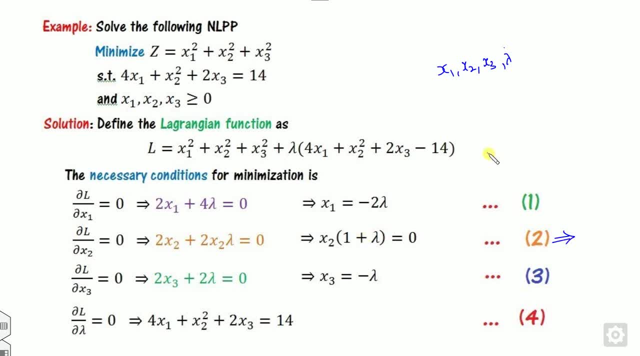 and lambda. so from second what you got, that is, either x2 will be 0 or lambda is minus 1 from the second. if lambda is minus 1, then what is the value of the x1 is this is 2. what is the value of the x3 is 1.. 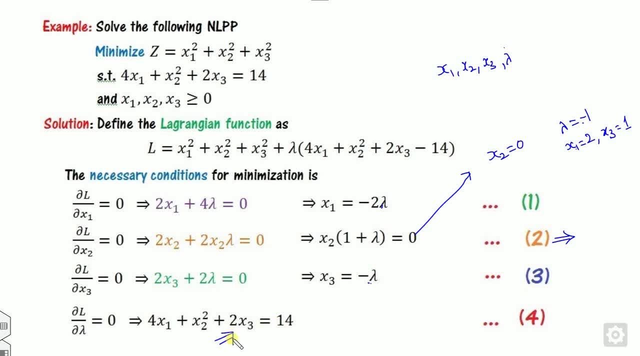 So if we substitute the value of x1 and x3 in here, we can get the value of x2. on the other hand, when x2 will be 0, we can see from here what will happen is 4x1 plus 2x2 is equal. 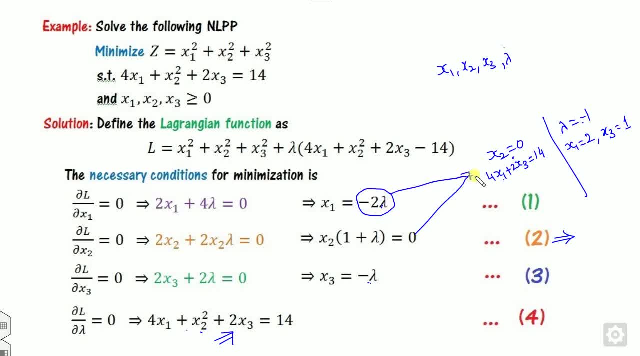 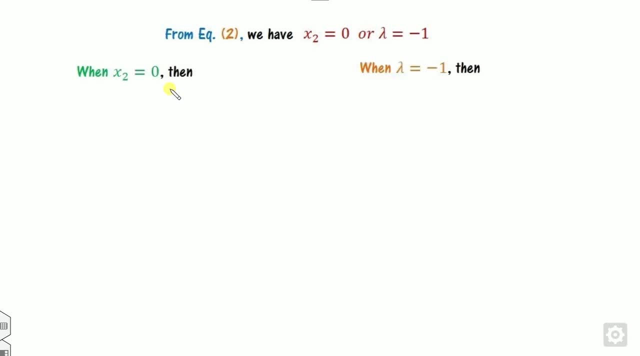 to 14. we can substitute the value of x1 in here. x2 will be here. we can find them. so look at that. this is the case. now. there will be the two case when x2 will be 0. we can get this expression. we can substitute the value of here. 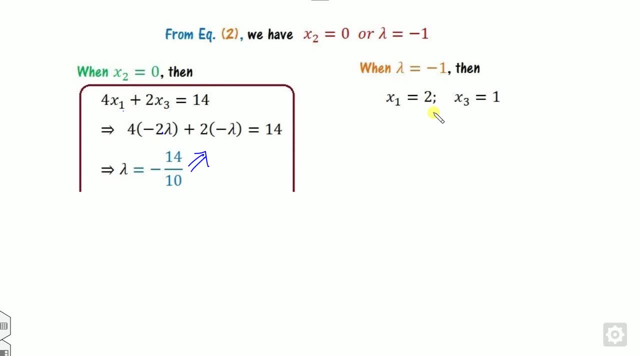 So if x1 and x2, we can this value on the other hand here. so this: it means we can get the value of x1 and x2. this and from this case now, this is a plus minus of 2, but it is given that x2 is greater than 0, so therefore the negative part will be discard. so what? 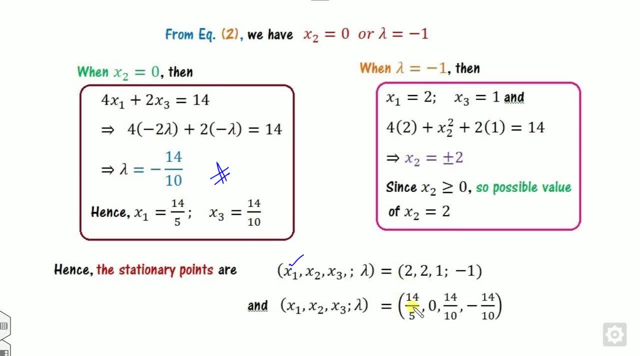 are the stationary point in this case, what are? the stationary point is: x1 will be my 14 by 5, x2 will be my 0, x3 is my 14 by 10, x4- lambda is here and similarly for this. Now these two points are there, We will check which one is the maximum and 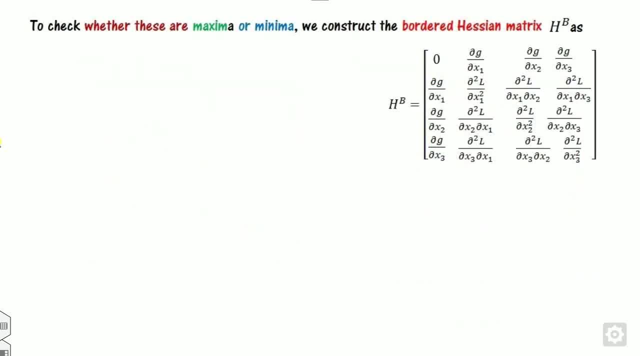 which one is the minimum. How we can check, We will draw the Hessian matrix, that is the border Hessian matrix. Then in this case you are not only check for the convex or concave. Why? Because the constraint is my nonlinear, because x2 square is there. So how you define that, Look at that. 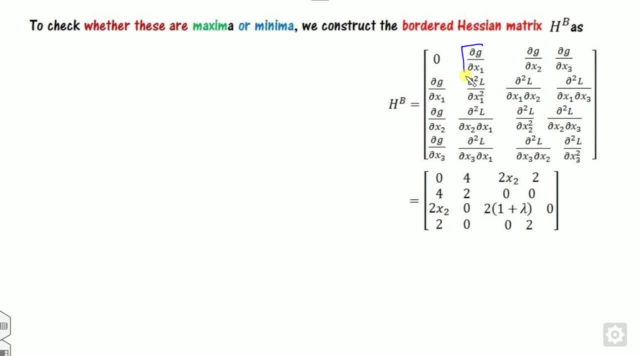 my function is here. You can calculate the value of this g. It will be here, because what is my g? This is nothing, but my 4x1 square plus x2, square plus 2x2 is equal to 14, something. So what is the? 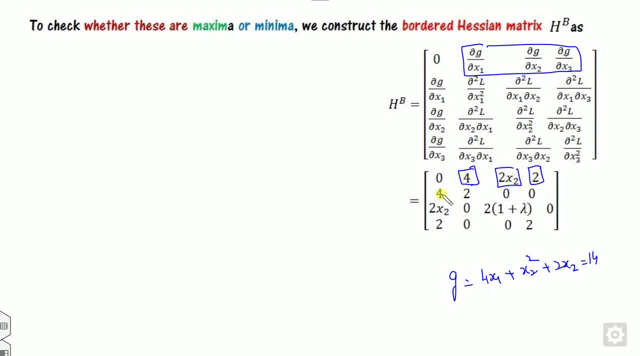 partial derivative of x1 is 4.. This is 2x2 and here, and this is the transpose, and once you define the l, you can take the derivative. Now there are the two stationary points and since this is 4 by 4, how many principal minor you will check- You can see that you can take the derivative of x1. 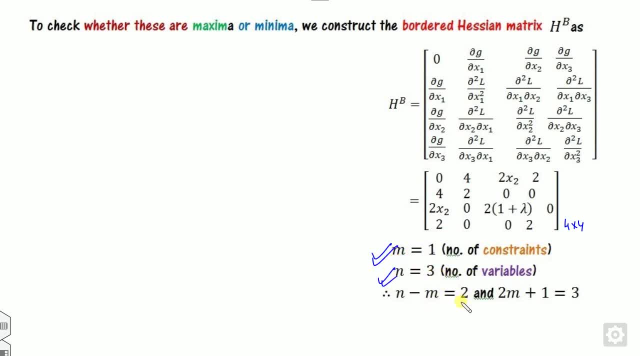 m is my 1, n is the number of variable 3.. So we need to calculate the two principal minors, but starting from 2m plus 1, 3, that is, we will check the d3 and d4.. So we will start the first. 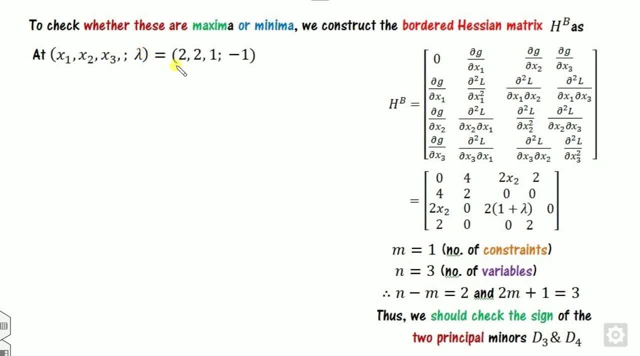 principal minus, that is, d3 and d4.. Now, since the first stationary point is this, we can substitute this value in here. Look at that: the value of the x2.. Now, this is 4. lambda is my minus 1.. So 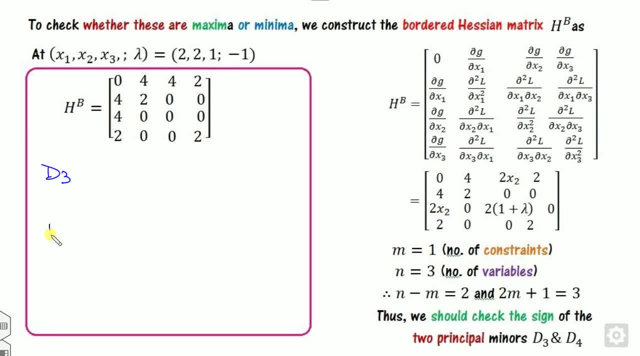 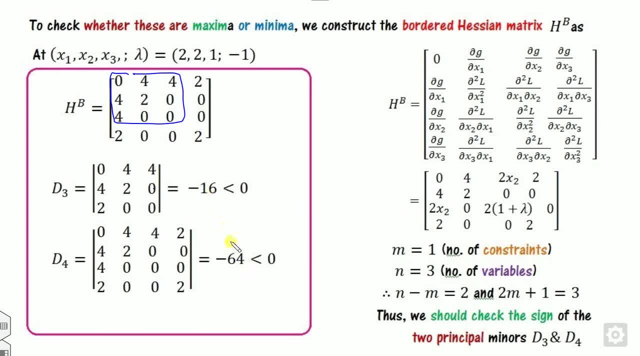 we will get here. So here we will calculate the d3 and d4.. This is my d3 and d4 and now you can see both are the negative. So you can check, since we are using the border ratio matrix. So we can see this point is minimum. 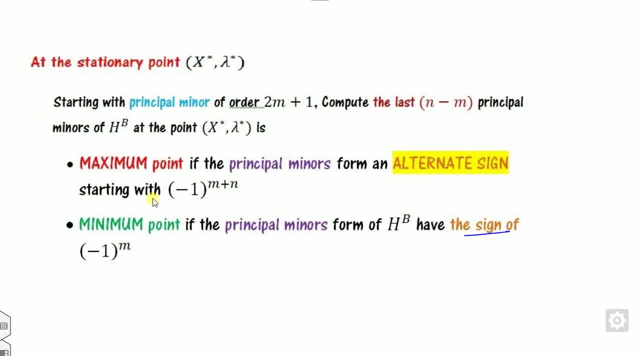 Why You can see they have the alternating sign is not be there. They are all the same sign. So since they are the same sign and the sign will be minus 1, m is my 1. that is a negative. So all have the negative sign. So this point is my minimum. 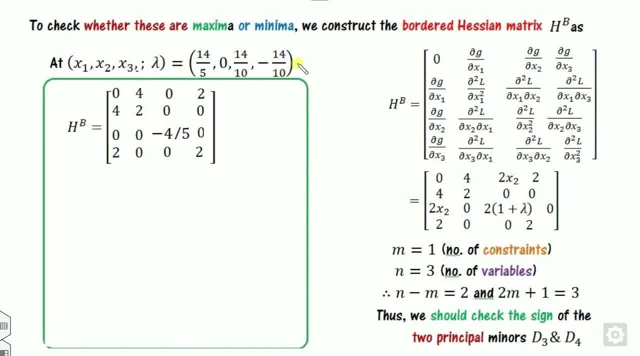 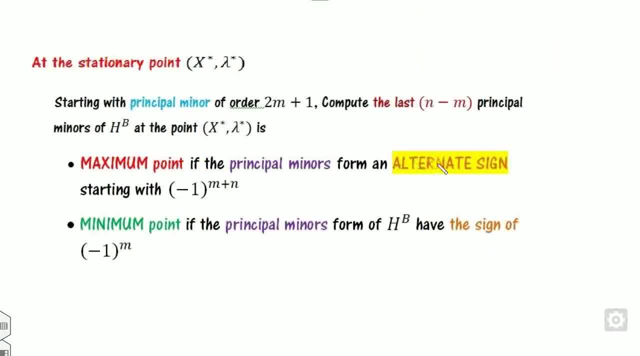 Similarly, we can check for the second point. At this point we can substitute the value here, because this involves x2 and lambda. Again, we will calculate the d3 and d4.. Now you can see. they are the alternating sign. Once they are alternating sign, can it be the maximum You can? 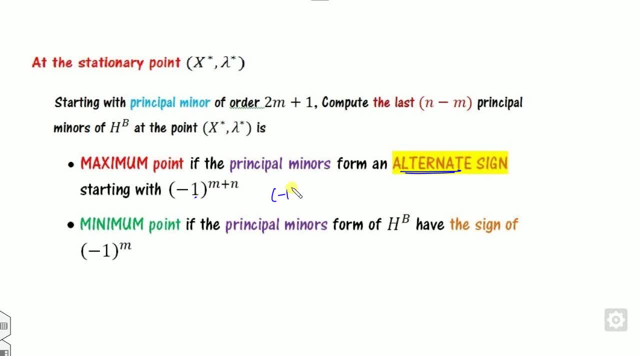 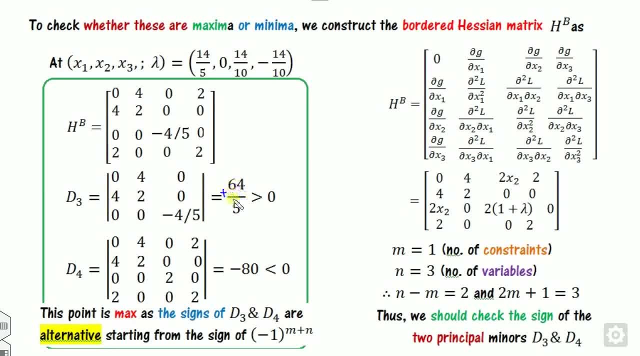 see if they are alternating sign. they will start from minus 1.. What is the m is 1 and is my 3. So that is a plus sign. So it will start from plus 1.. So it means this is the. 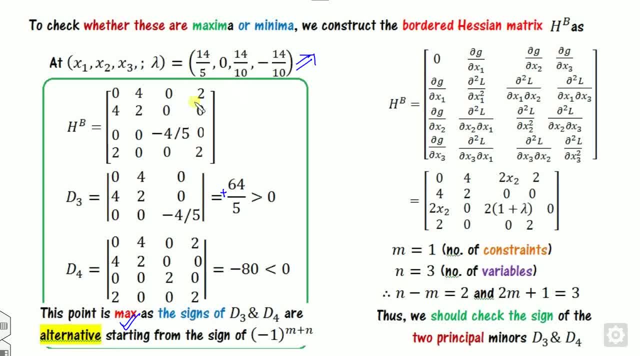 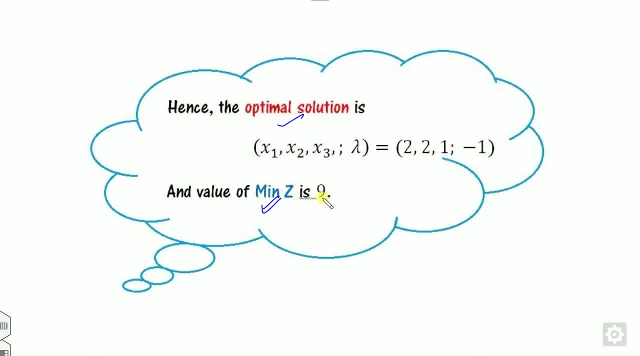 maximum. Hence this rationed point gives the maximum value. Other value is the minimum value. Look at the last example. So the optimal solution says: my problem is minimization. So it will give you a here. Look at the last example. What is the given statement is a: 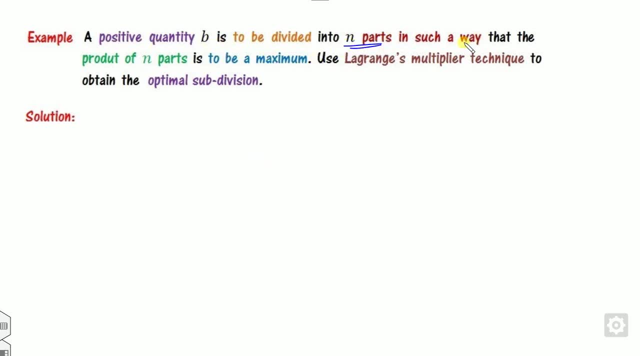 positive quantity b is divided into the n parts. Such a way the product of the n is maximized. So you have to take, if I divide the elements into this, what is my objective function? You have to maximize their products. So that is x1,, x2 and up to xn. subject that: what is the 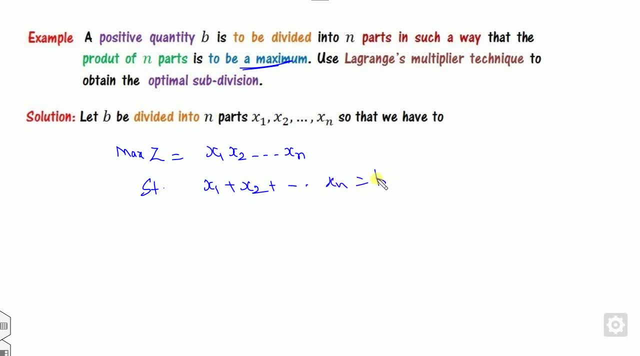 maximum sum of this will be b, And since all are my positive quantities, it is given that. So this is my LPP Again. you can see this: the constant is equality sign, So you have to firstly define this Lagrange multiplier. Once you are defining this, then how many variables are?